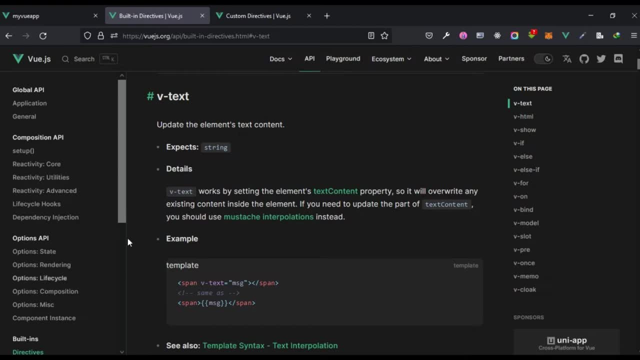 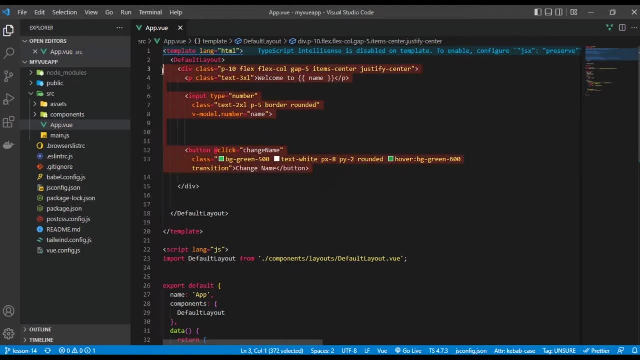 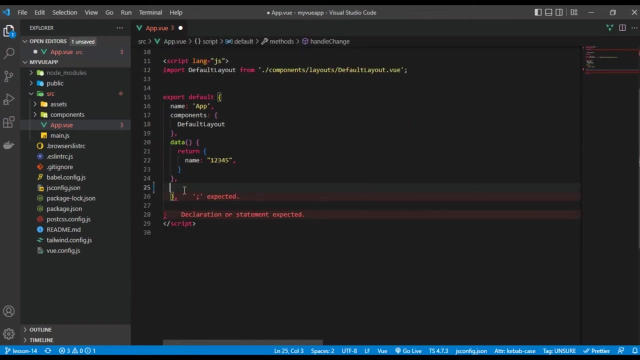 comments section below. okay, so, let's get started. the first one i'm going to show you is v4, and this is actually help us. so let's clear the previous code we have right here. this will actually help us to loop through and render dynamically, okay, so, let's, let's do something i'm going to okay. 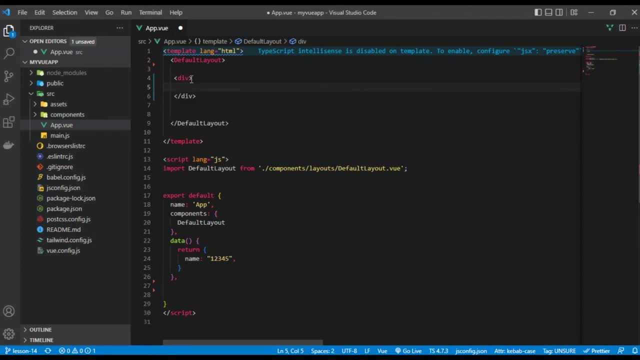 have my div tag and i just want to have okay, let's say um h3, which says okay, lists, and we're going to have a class of, I think, a class of text, very Excel and font boat. that's works fine and what I'm basically going to basically. 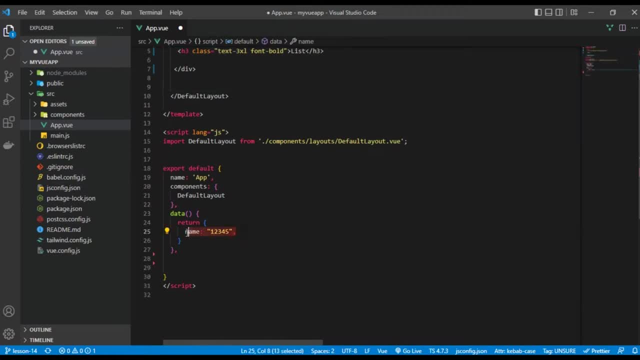 going to do is I'm going to return a value which is going to be, let's say, data, data lists, and then it's going to be an array of objects. okay, so the object is going to have an ID of, let's say one, and then, basically, it's going to 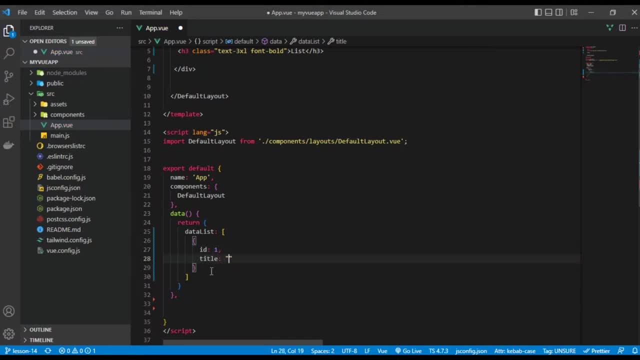 have title of least one, and then it's going to have, let's say, active, and then it's going to be false. all right, so you basically going to have something like this, and I'm going to skip ahead where I'm going to complete this and have about 12 object in this array, okay, so I 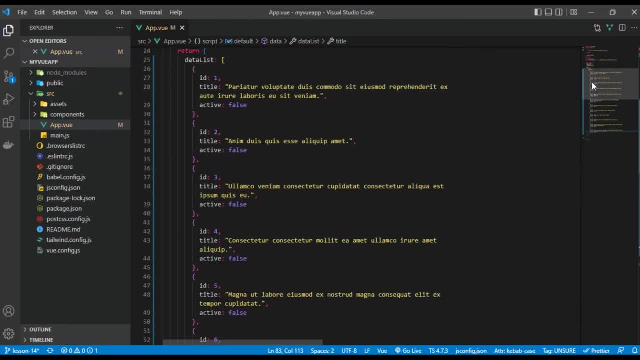 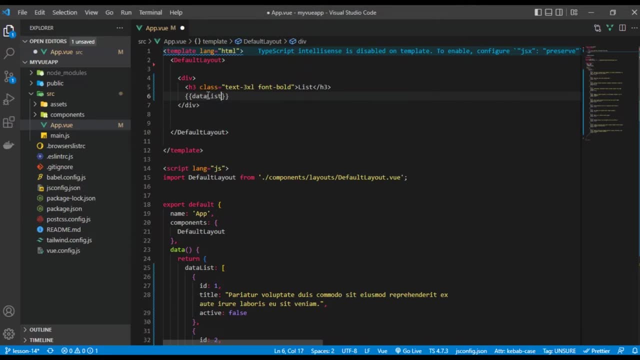 basically have 12 objects right inside of this array and we can basically look at it like data lists and let's save that. and let's come back to our application. oh, we can see, it's right here. that's definitely interesting, and I can just have another div right here and this: 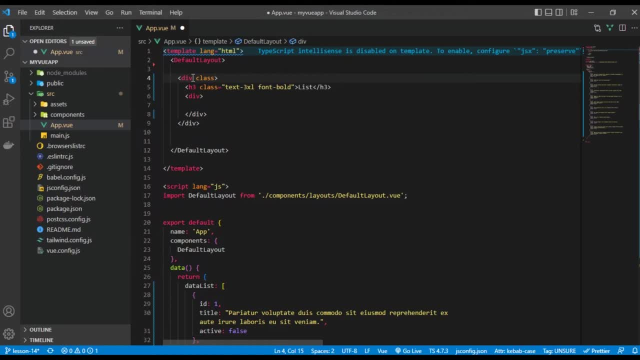 is going to be: have a class of against, have a class of max width and let's say, 500 pixels of 100 pixels- no, I think 1,000 should be okay, and then MX auto okay, and this should be text center and yeah, should have once it's to actually. 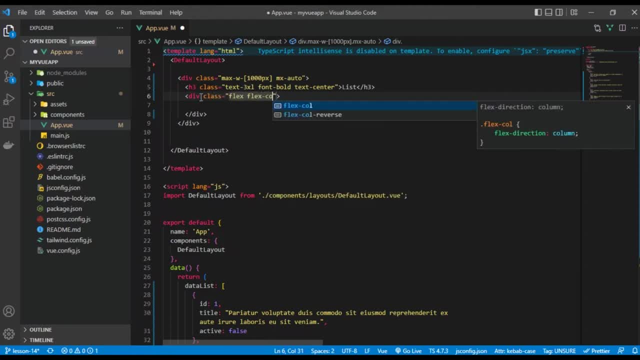 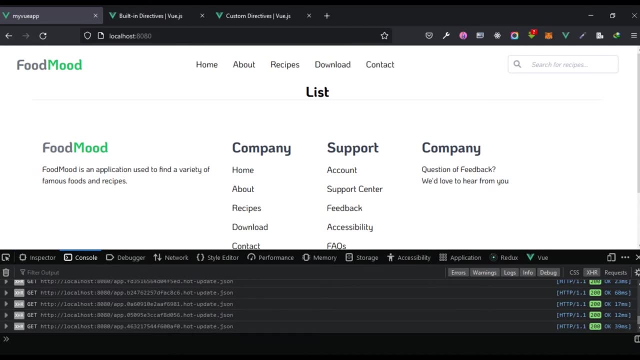 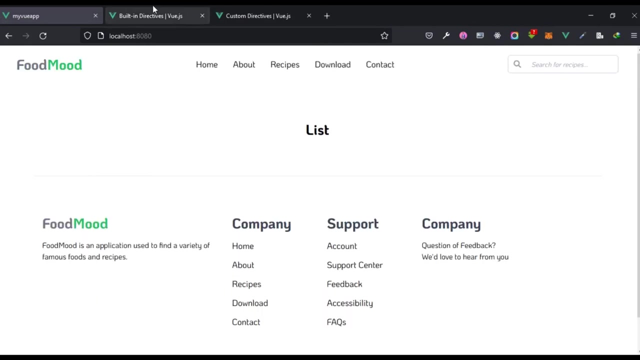 have a class of flex, flex coal and then gap five, and okay, this is basically what i want. okay, we have something like this and let's add a bit of padding. okay, and we have this. i want to actually render our list right here, okay, so let me close this and want to render our list using one of 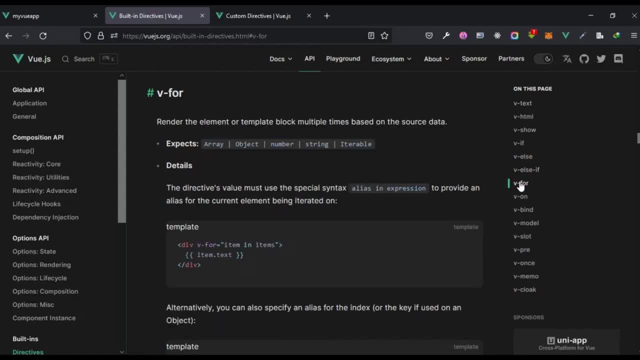 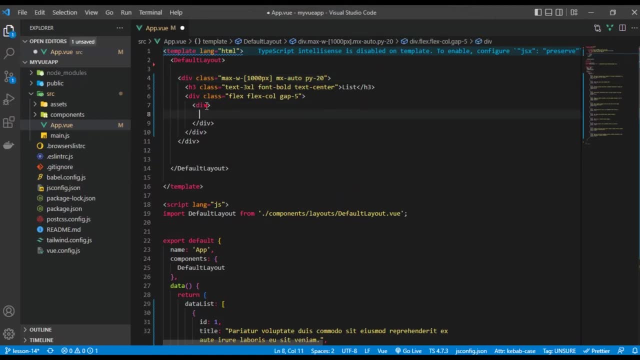 these built-in directive, and the first is i'm going to use this v4. so, basically, i want to render each one of these into each of their div tags, and what i'm going to do is i'm basically going to have v4 now, using the extension that we installed earlier. it will actually give you um, you see. 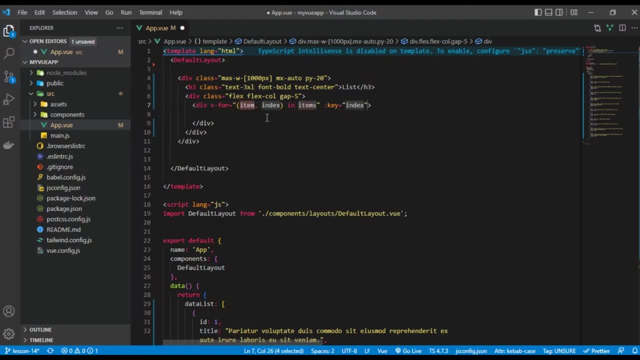 it brings the suggestion right here. so i'm basically going to use this syntax here. so we want to actually access this. look through this particular as well elements. so, uh, this particular data rather. so we say item index in data list and the key is going to be indexed. so basically we can access this right here, the all of the single object that we. 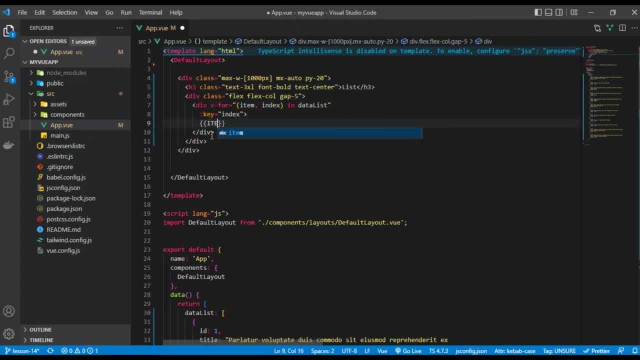 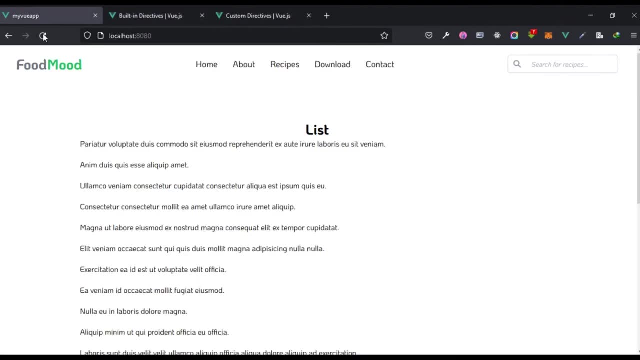 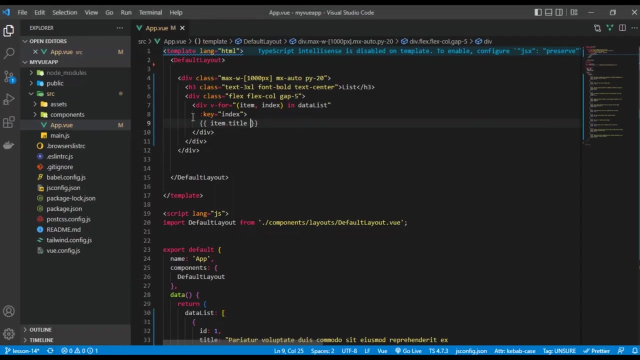 have here. so the way i'm going to do that is i'm going to say item: okay, item dot title. let's save that and let's see what we have. okay, so we can see it actually gave us and rendered each of the lists right here, which actually makes a whole lot of sense because it's and it actually reduces the amount of code. 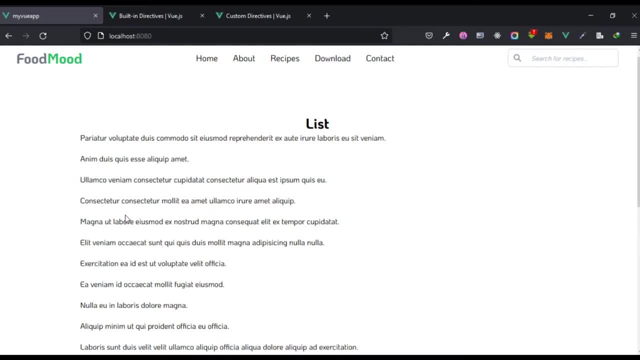 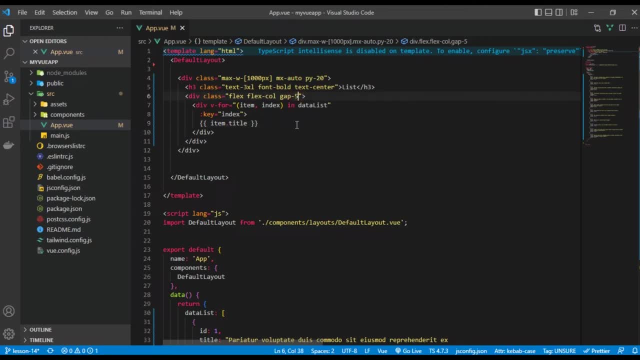 and we are able to dynamically output a particular element, a particular template, etc. using this v4 directive, and let's actually make it text center. um, okay, let's see 10. and let's see, okay, we have all of these now. this works fine and this actually works well. so what about? let's say, um, 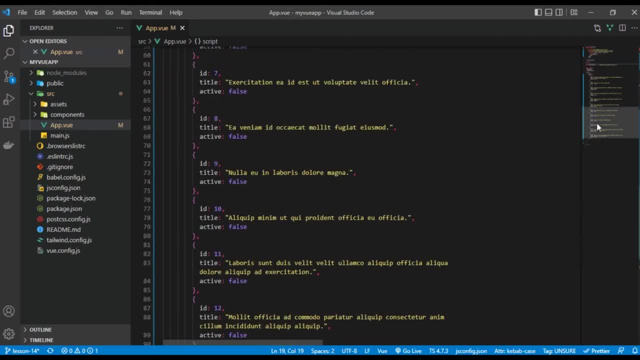 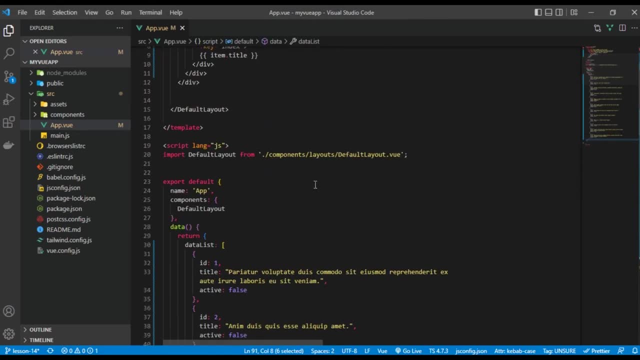 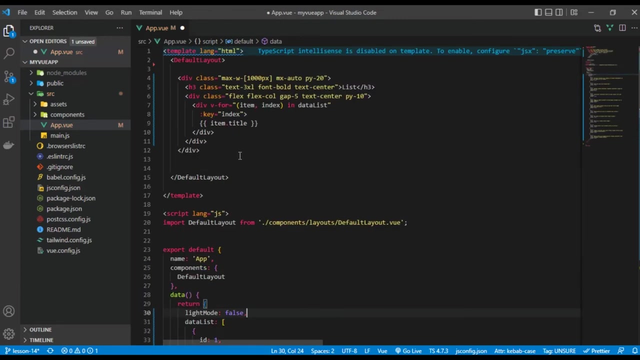 we do. we do something or something interesting. let's say, we have another data right here and this is- let me just put it here- okay, this is, let's say: um, okay, let's say we have light mode and then this is false. okay, now we can basically come down right here and we can have a click event. 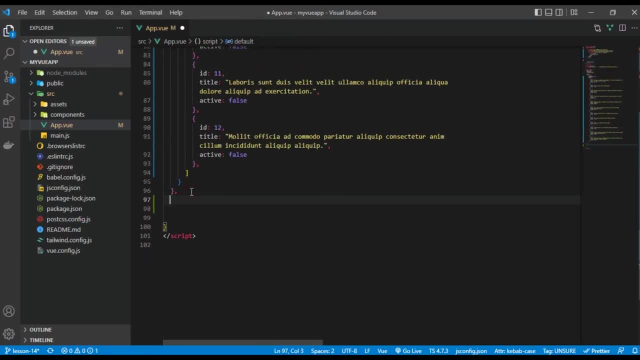 and it's going to basically say: okay, so let's have our click events here, i'm going to scoot this in. so let's say let's close this. um, yeah, so let's have our method array method. and then this is basically going to say of this and i'm going to create change. okay, switch. 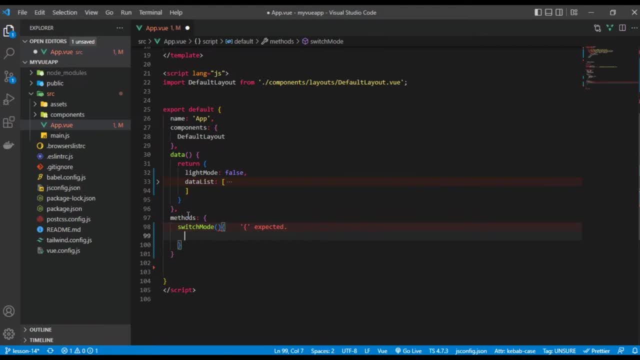 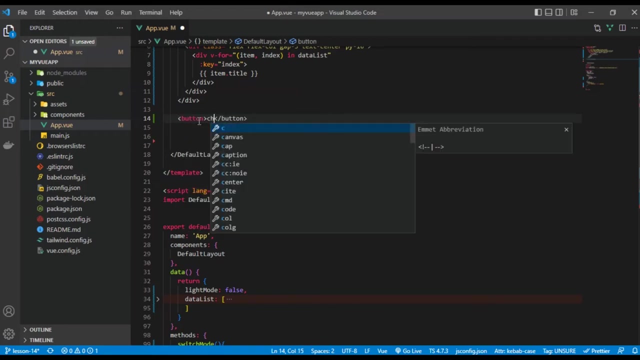 mode. and let's see, it's going to say this dot light mode is equals to not this dot light mode. all right, and we're basically going to have a button. nothing fancy, i just want an irregular button change and then this is going to have at click and then it's going to be equal to switch. 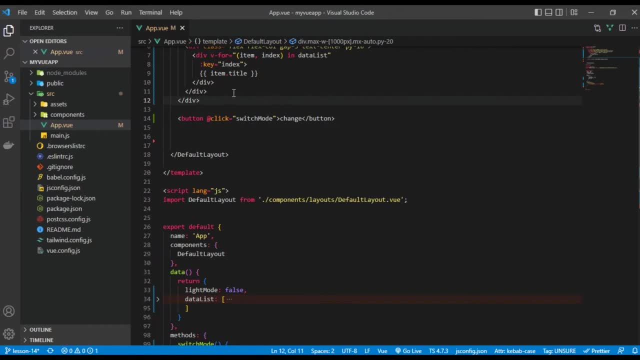 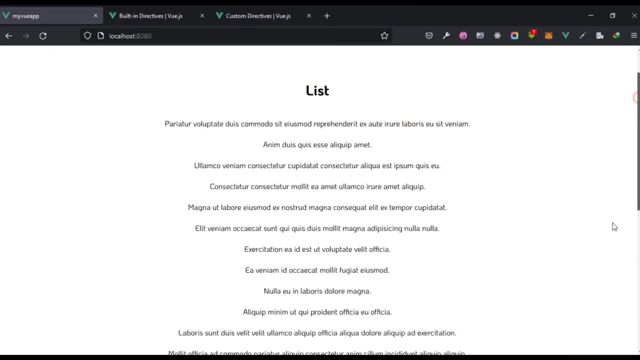 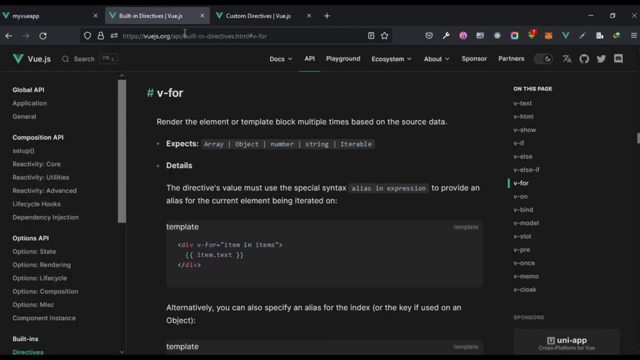 mode. all right, what we basically want to do is: let's output this here: light mode. now, what we basically want to do is, whenever we click on this- okay, this, currently it is false, but whenever it is true, we are going to dynamically render using one of these views in directive, which is if and else, yeah, so basically, what i'm going to do is: 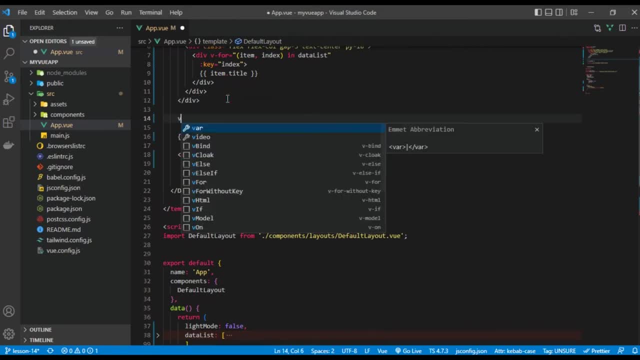 something like down here i'm going to say, um, i'm going to have my div and i'm going to say light mode, and then, right here, i'm going to say dark mode. so what i'm basically going to say is v, and then if, and then let's auto generate that. 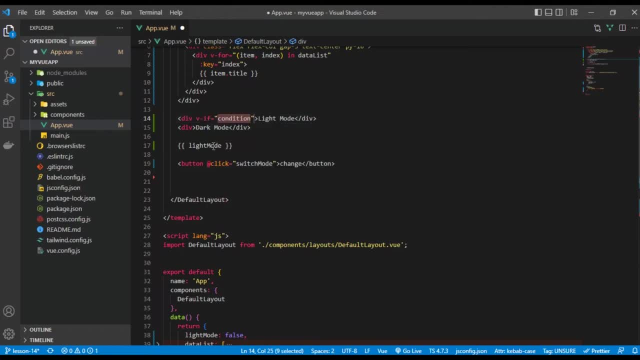 okay, so v. if so, if the light mode is actually true, we want it to render light mode, and then we're going to add a class of um, let's say bg, green, and then padding of five, and then text white, white, okay, but we're going to say v else. 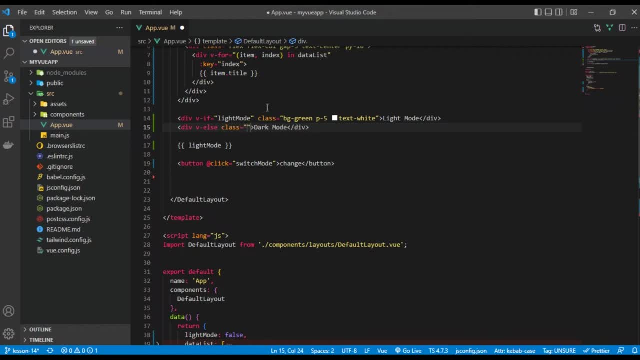 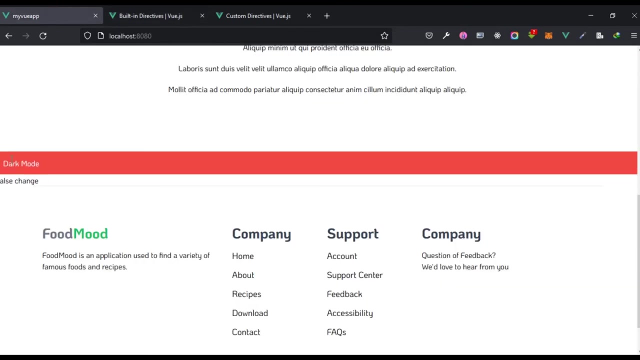 okay, this is going to render and then this is going to have a class of bg: red, i think 500- okay, this should be like 500- and padding of laser's three pixels and text white. okay, so let's save that and let's what that is going to actually give us. all right, we have dark mode here now, if i should click on. 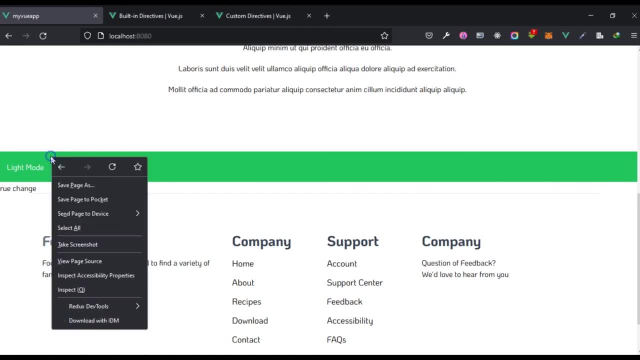 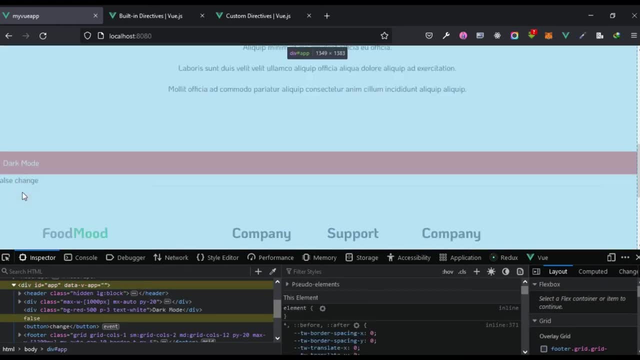 this. we see it's rendered this, and it's not just we are changing attributes or something. if i should inspect this, we can see this particular element is being rendered. or if i should click on change, that particular element has been taken away from the dom. so that is one of the building directives. 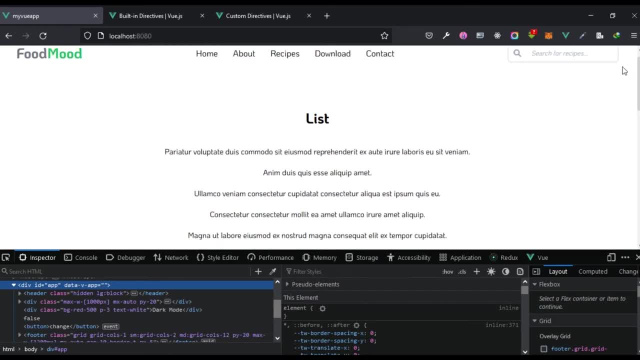 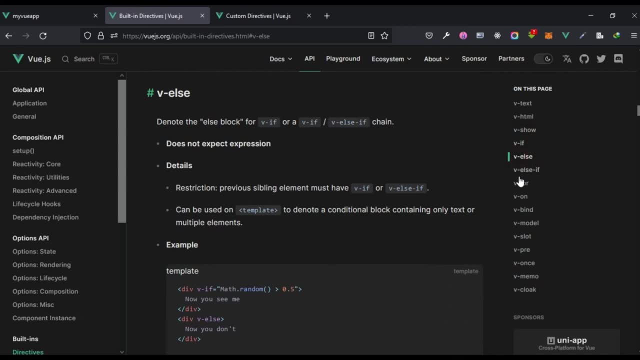 that we can use. okay, finally, let's give ourselves a task with this view directive. we see we have tons you can just explore with this, uh, and, as i mentioned earlier, the link to this will be in the description below. so let's kind of give ourselves a task where, whenever we click on each of these, 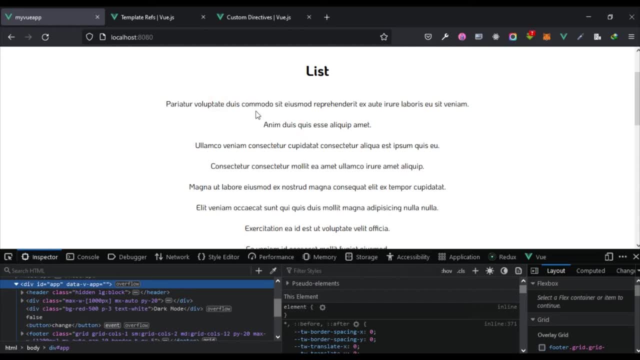 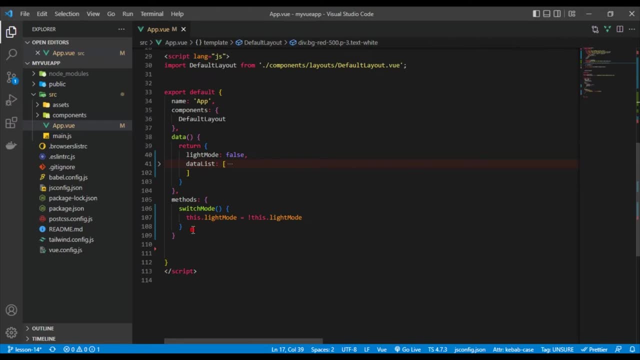 items, just like a to-do list. okay, something is going to happen, so basically let's kind of do that right now, and i'm going to actually have a click event which is going to say filter to do's and basically i'm going to take in a parameter which is id. i think we have id. yeah, i'm going to take in the id. 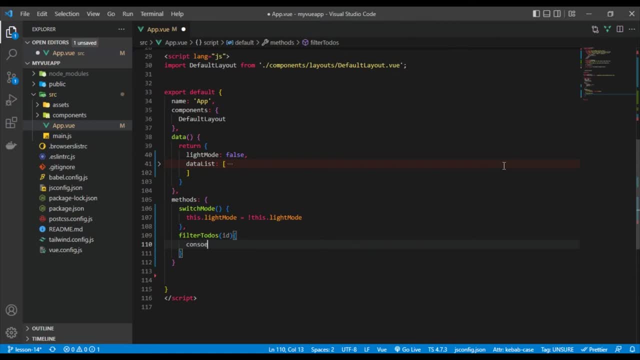 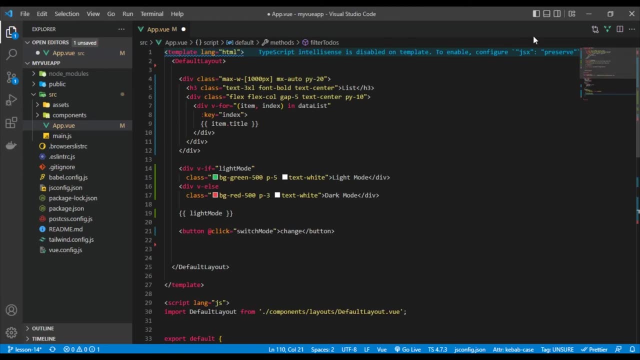 all right, and i'm going to consolelog. let's first do this consolelog and then id, and what we'll do is attach the click events to each one of these. okay, um, at click, and we can do something, such as call this, this method, right here, and i'm going to say: 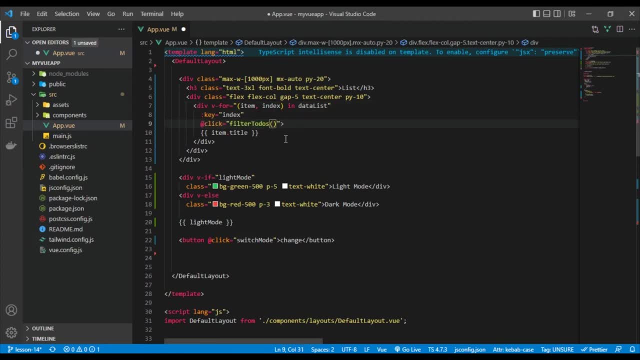 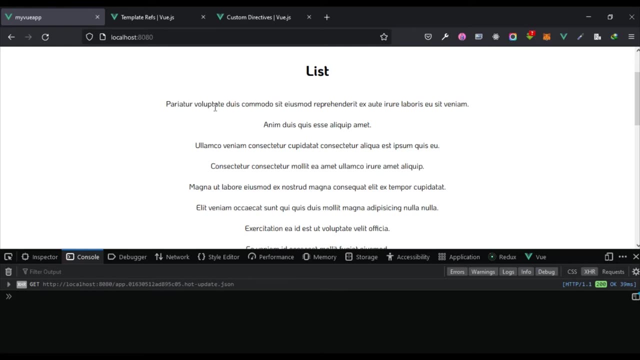 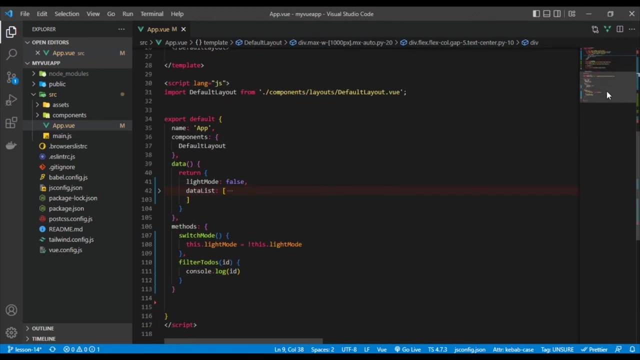 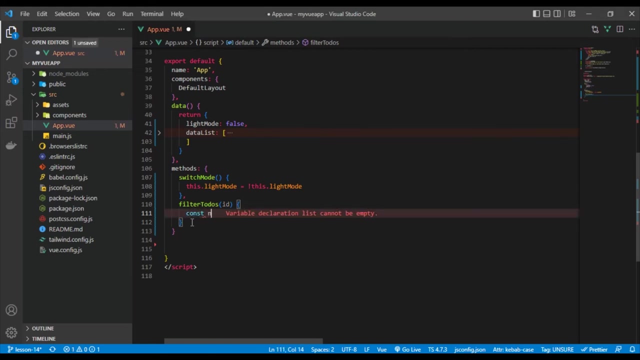 okay to do, filter to do's, and it's going to take in itemid, okay. so let's actually come to our console here and click on this and say one, two, three, four. so what we basically want to do now is: i'm going to say const, i'm going to say new. 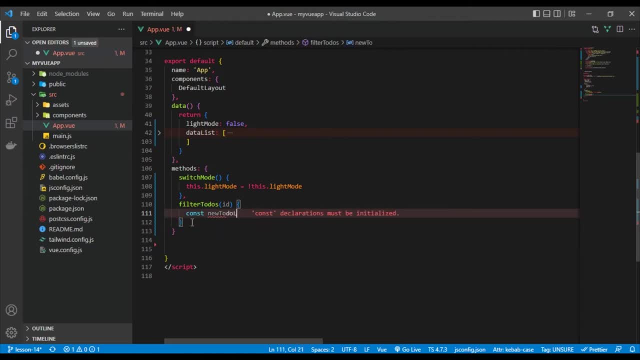 to do list equals to this dot data list, dot filter, and basically it's going to take in list and it's going to say, um list, dot id is not equals to id. and then what i'm going to say is: this dot data list is equal to new to do list. and this is it very simple, okay. 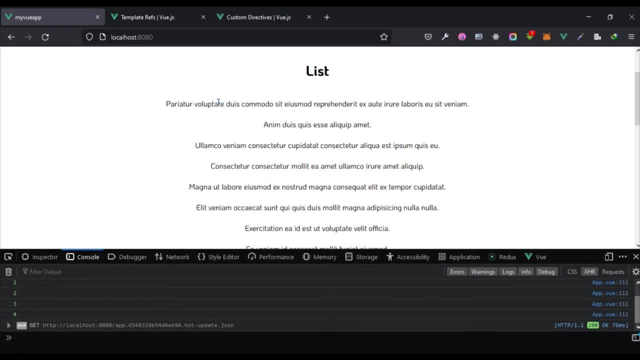 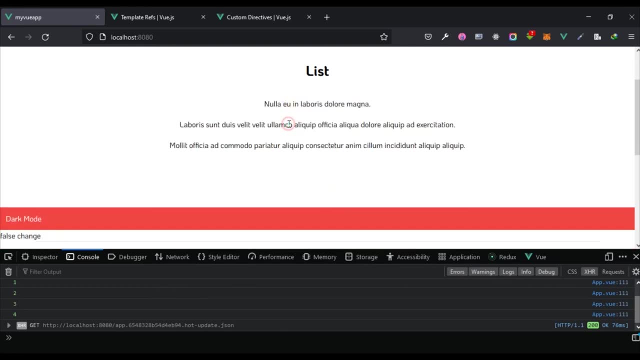 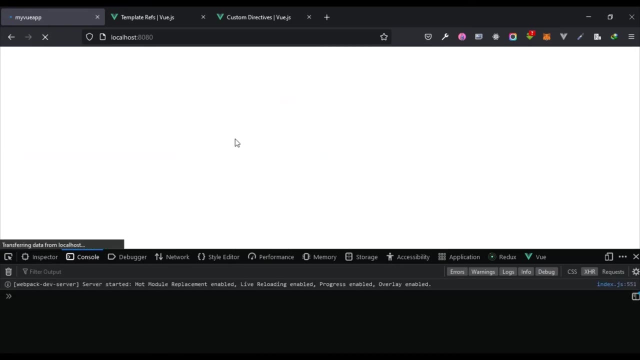 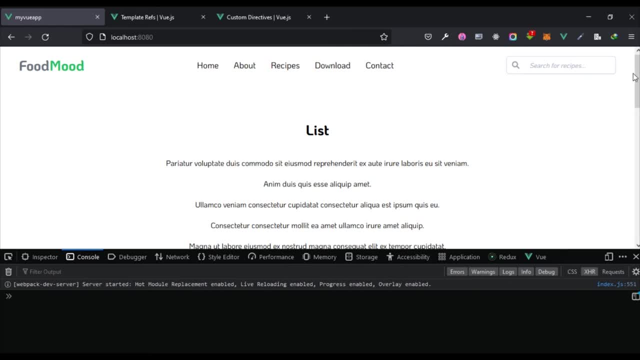 uh, i kind of want to give you a a challenge before we continue. okay, try and do this by yourself. create a new app and then have an input field. so i just want you to combine everything that we've linked so far with directives, but data binding and every other thing- events combine. 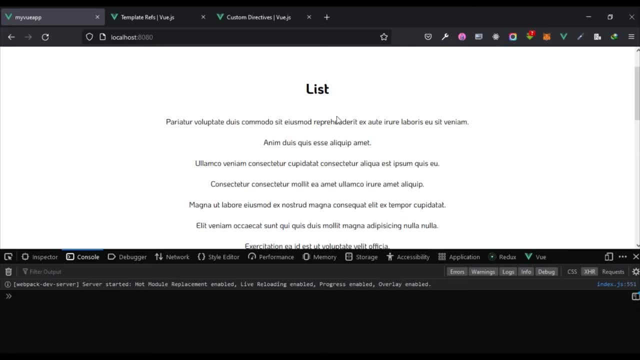 it and try and create a to-do list where you can basically have an input and a button that adds to the list and you can basically click on one of the item or maybe a button beside and it's essentially just removes that from the list. so how about we actually go into custom? 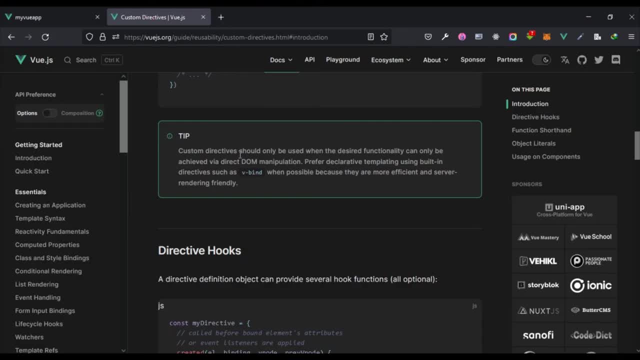 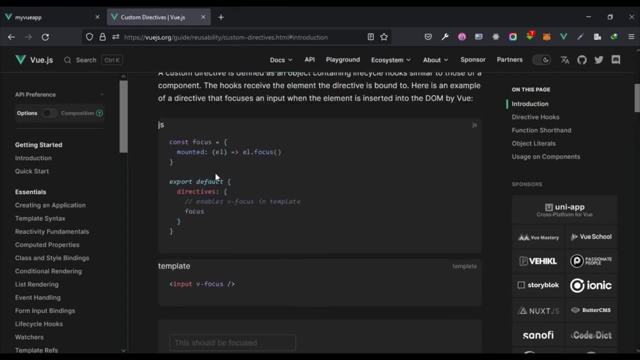 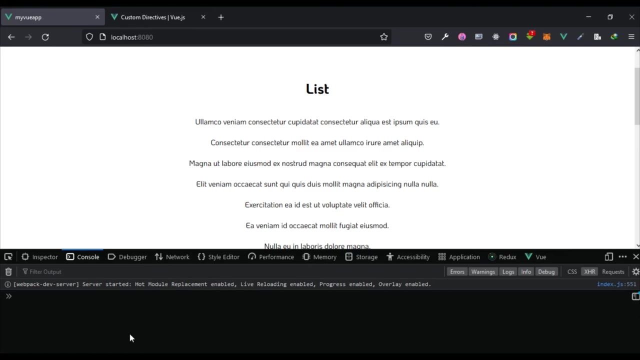 directive and if we should come here to view js documentation. here i think they have a very simply simplified example, which is this: okay, we can basically have a function aha that says this: okay, let me implement this, that i'm basically going to come here and let's um, just come here and let's see, i'm 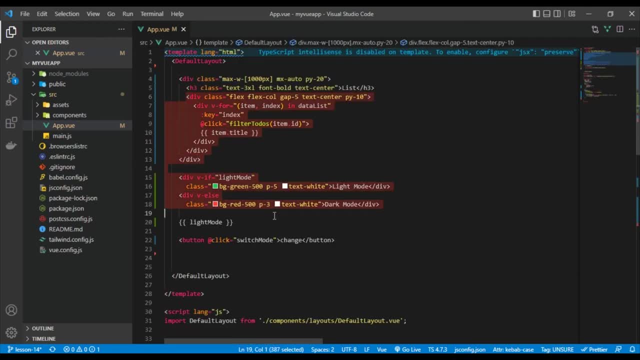 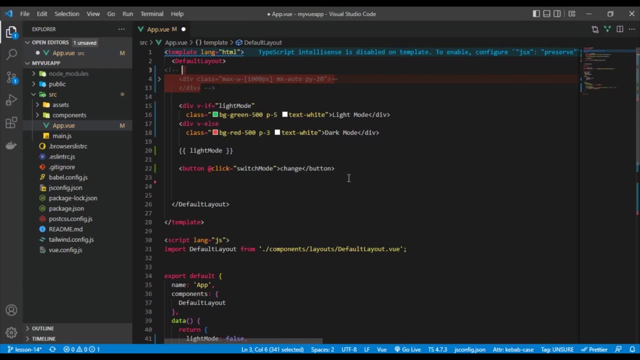 going to comment this out. okay, i'm going to comment all this. so let's comment this out. and comment this out also. and what i'm going to do is i'm going to have a div and i'm going to have an input, and the input is going to have a class. let's say class. 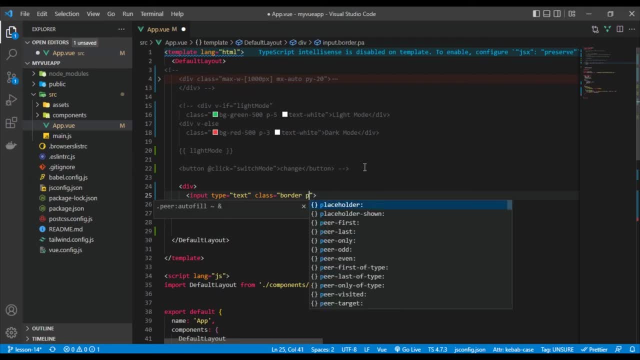 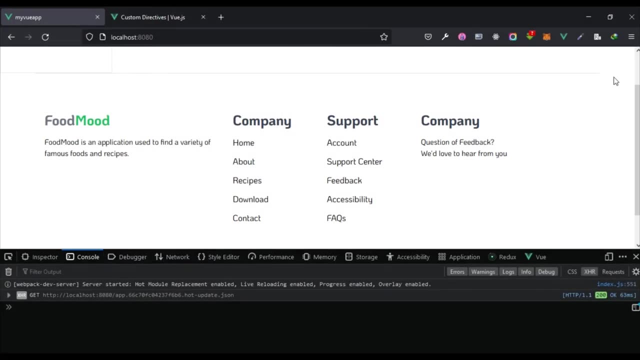 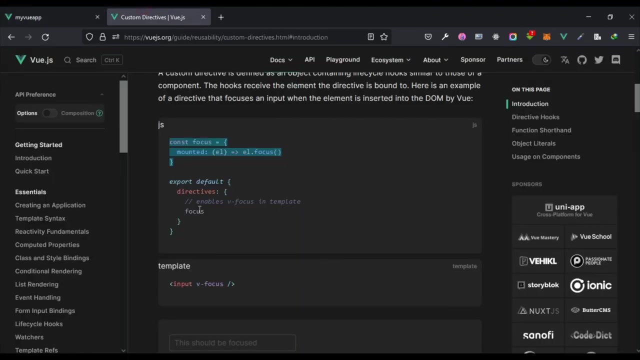 of. i just want to have a border and padding of five. okay, that's just all i need for now. and coming back here, okay, we should be able to see our input somewhere, somewhere here, which is fine and well. so what? the goal of this is basically to have a to. 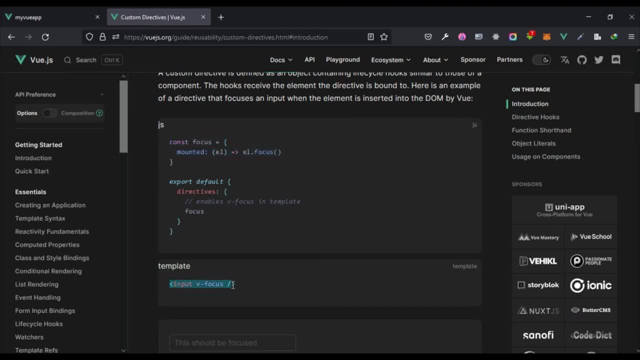 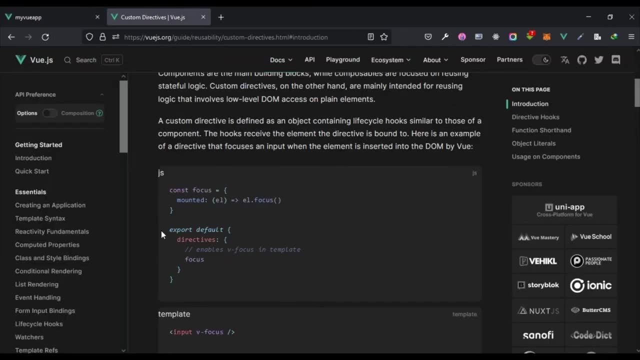 create a um custom directive which is v focus, that whenever we add it, automatically it's going to focus in this input field here. okay, so the first thing i want to do is i want to see if we need to create a Deus orbit that we want to use there, because i buy that to a shift code ofномon Прgle. So first thing, 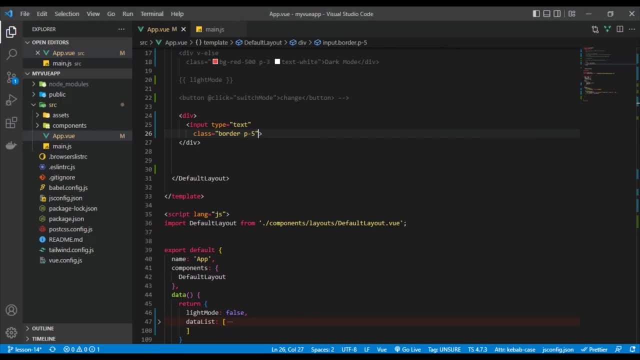 what i want to do. i want to do: i want to order in that these inputs and expected returns and if someone or you have a specific comp plan, okay, that's going to add it to the different units and do is. i'm going to come right here back to my code and we're going to make a bit of manual adjusting. 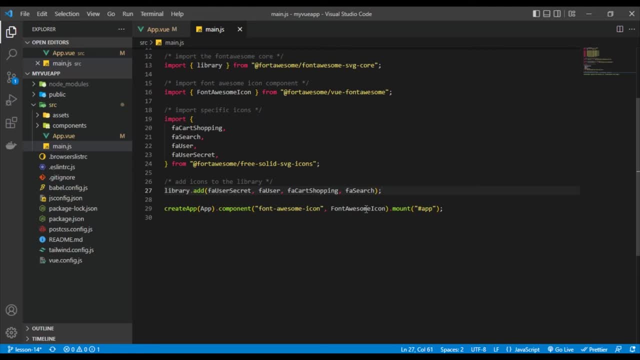 now note: if you're actually running your app right now, you might need to quickly pause the development server, and what i'm going to do is i'm going to create a new variable and it's going to be equals to create app. so i'm just going to um reconfigure the app structure right here, so i'm 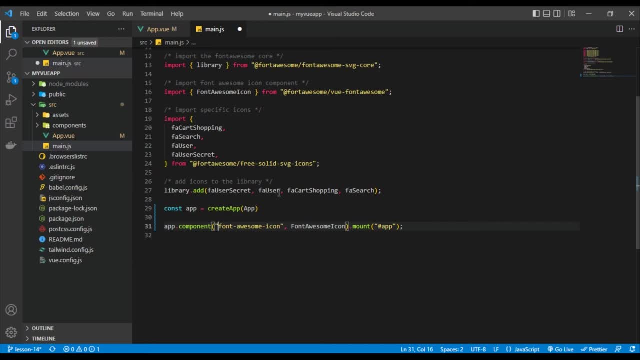 going to then say app dot component. so this basically still translates to what we did here, but we also get the ability to actually tap into up dot directive, okay. so this is basically going to take in a string the name of our directive. i want it to be focus and we are basically going. 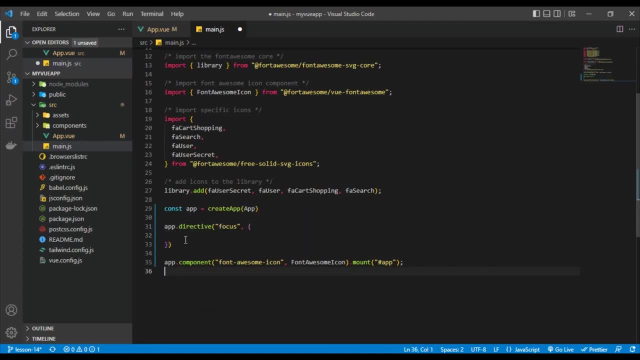 to have this right here and we can tap into various um life cycle. now we're going to go into lifecycle run, so you're going to go into gameplay. activefaq济 2ft- deepfai- we're going to go into in the next lesson, so don't worry too much about life cycle. so what we are going to do is mounted. 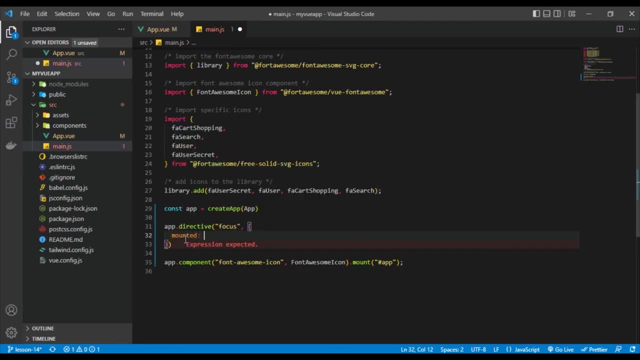 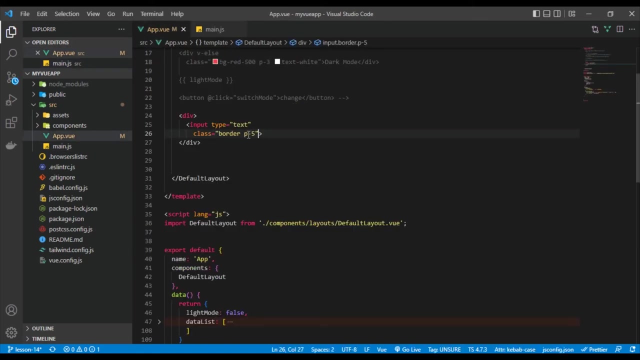 okay, and then we're going to have: okay, it's going to take in the element, and then I'm going to return element dot focus. okay, that's basically what I want to do and I'm going to save these and I'm going to just say: V focus, all right. so let's save that and let me restart my development server. okay. 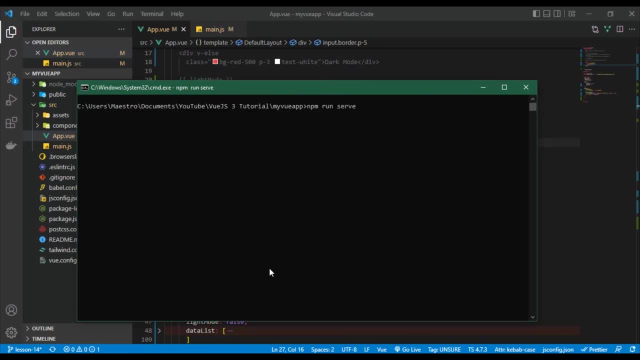 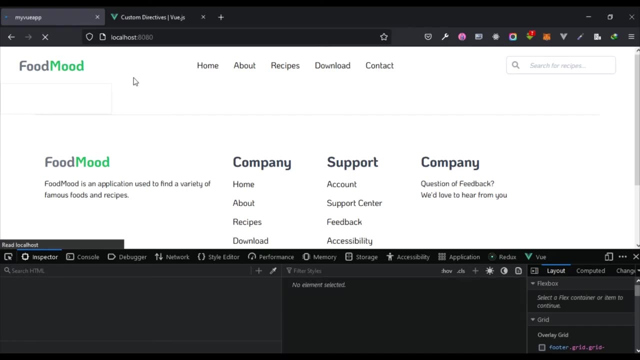 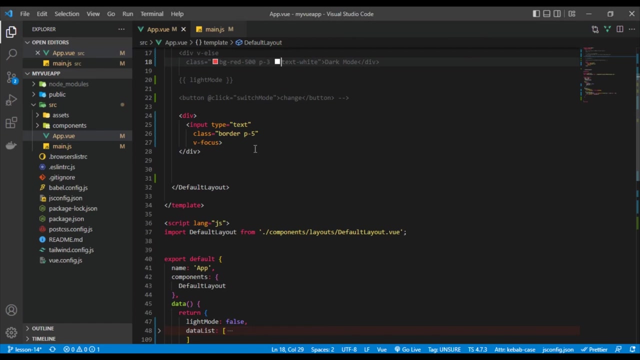 so I'm going to restart this and then run it again. so let's come back to our hop right here and we can automatically see that being focused. so let's, in case you're not sure, let's actually create another custom directive which would automatically let's. 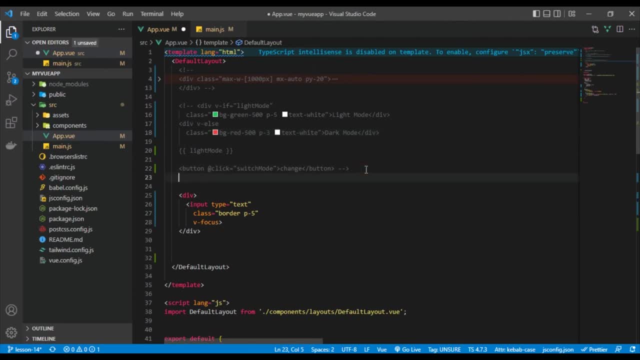 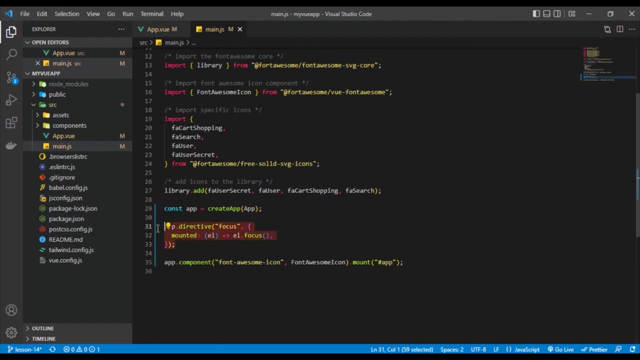 say increase font size. so I'm going to put here, I'm going to create a P and I'm going to say font increased font size. and we're going to create another app directive and this is going to be, let's say, um fee big. and then this is going to say: element dot font size. 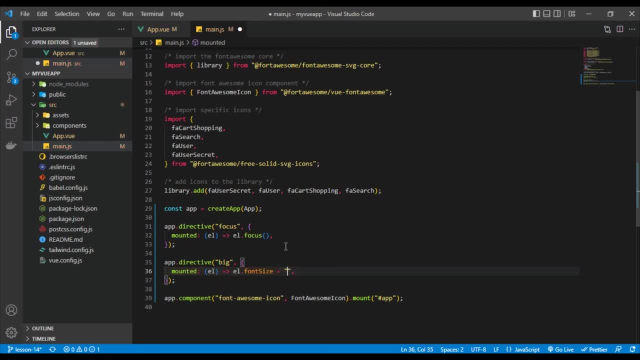 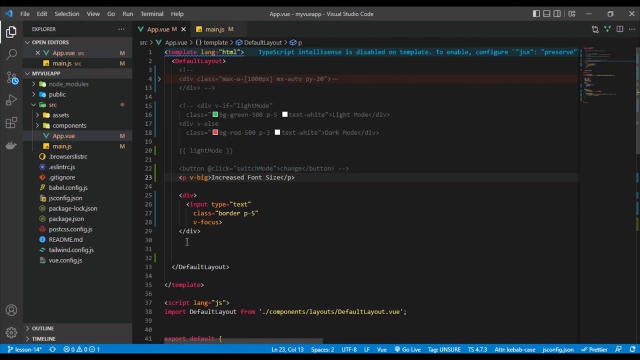 then is it going to be, let's say, um 100 pixels. okay, so let's save this and we can see the um, this particular element, right here. so what would happen if I should come here and I should do something like V big? let's see um if that would work. and no, it's not working. 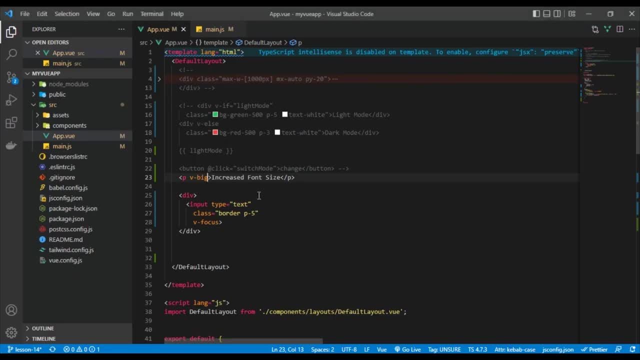 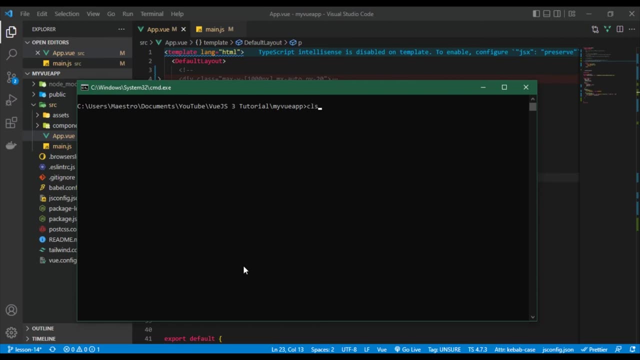 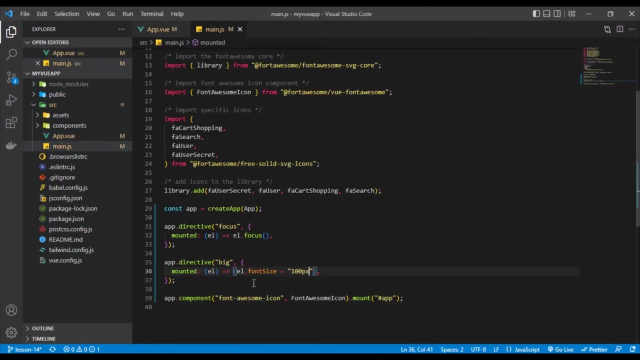 so I'm just going to restart my development server, okay, so let's do that, and I'm going to run it again. okay, but I think there might have been a mistake here, so let's actually had style. okay, this should be dot style, dot font size. okay, so let's see, did that work? 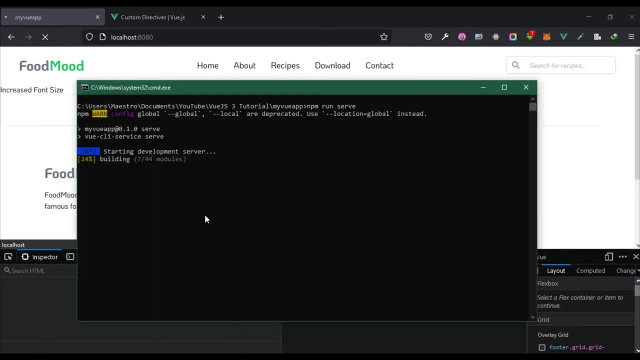 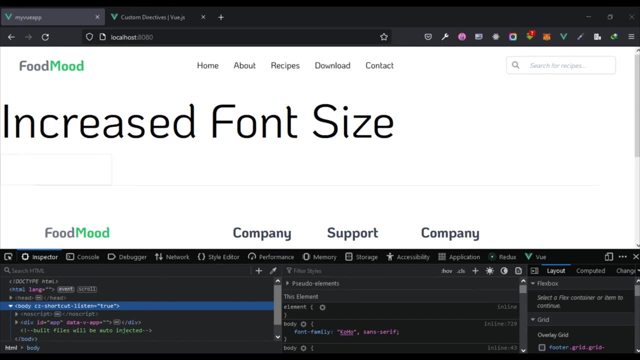 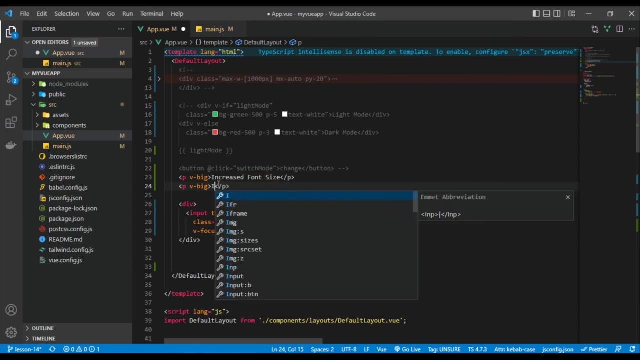 okay, our development server is still starting up, okay, so let's go back to our app. we can see this as increased font size, so that automatically is going to apply to this. if I should have another um paragraph here- and I should do maybe have um, something else- let's just use a div and we say: okay, adjusted font size, and I can just put V big.